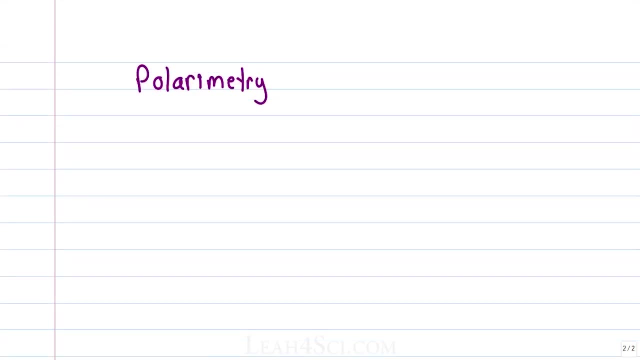 light in either direction, Which brings us to polarimetry. Polarimetry is how we measure optical activity, but the actual device is called a polarimeter And if you look at the word carefully, you get polar, which has to do with light, And meter, which has to do with measuring. Light, is how we 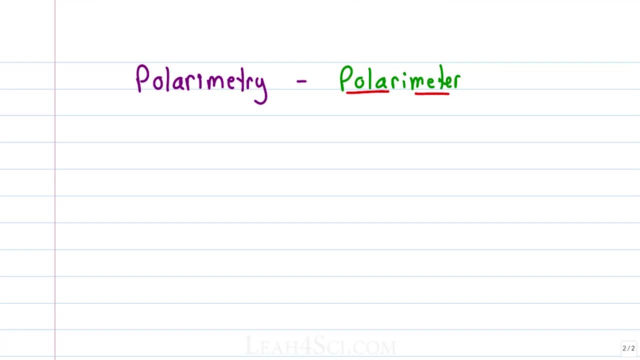 measure optical activity of chiral molecules. Think back to general chemistry or even physics When you learn the topic of plane polarized light. remember that light can exist as a particle or a wave and if we look at it as a wave, it oscillates up and down. up and down. 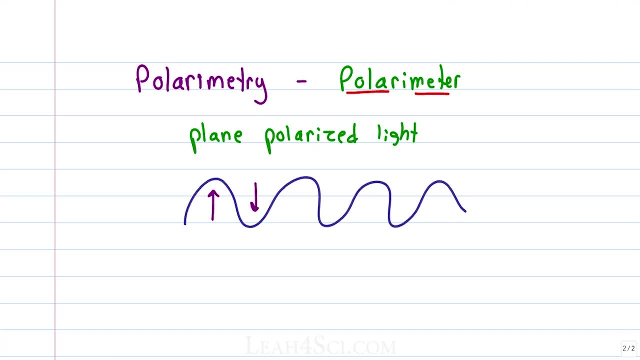 but in one direction. So notice here: it oscillates up and it oscillates down, But if we were to look at it head on, all we would see is straight up and down, and up and down, and that's in one direction. This is sometimes referred to as monochromatic light, because we're looking 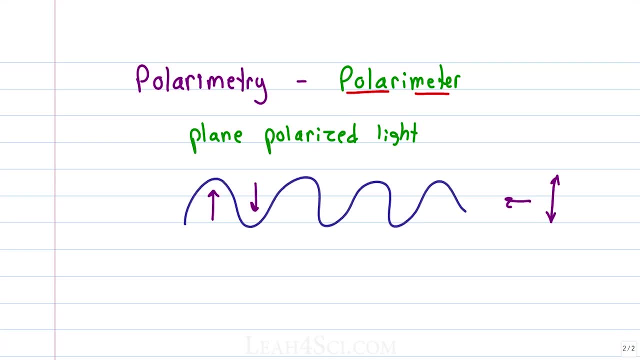 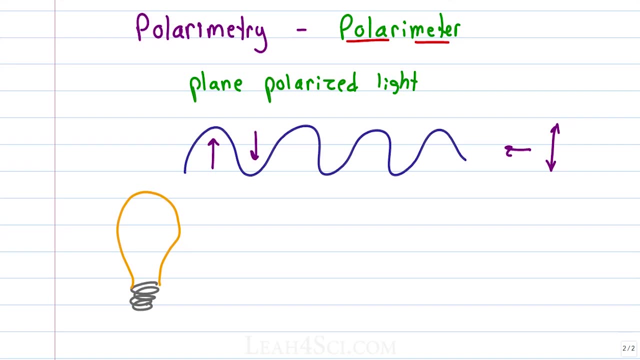 at light in one color and one wavelength. But if you look at something like a light bulb that is lighting up a room, it happens because the light waves are coming out in every direction, So each wave that's coming out is oscillating in one specific plane. but 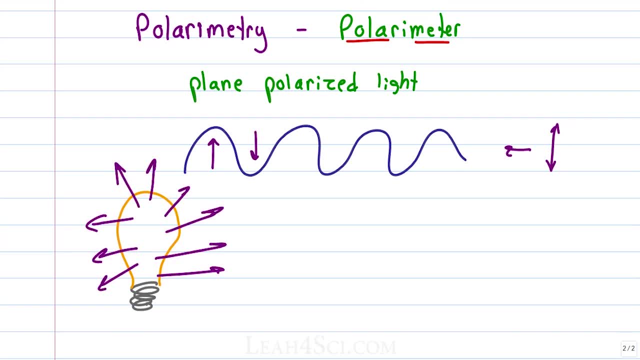 overall, the light is going in every direction and that's how it lights up a room. When we want to use light to measure optical activity, we need it to be going in one direction, because if it goes in one direction and something makes it turn, we can clearly see that turn. 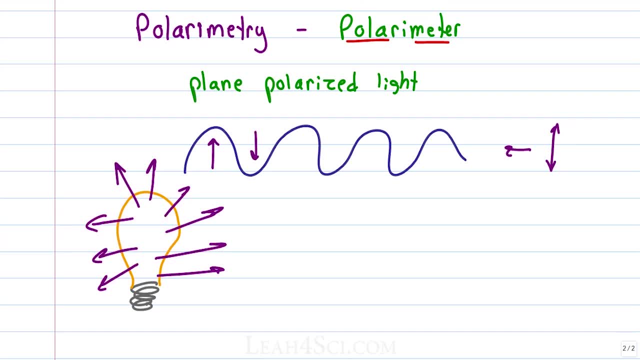 happening. But how do you get plain, polarized light in just one direction? What we need to do is place a filter in front of the light. So imagine that this is a filter that has a 41 annihilation sheets, a tiny little slit in one direction, So when the light is hitting it in every which way. 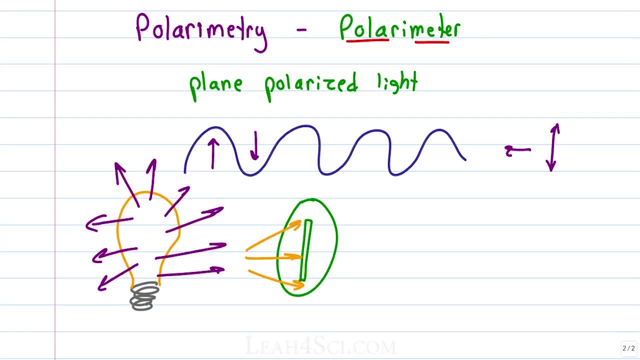 only the light oscillating up and down in the direction that allows it to pass through the filter is able to continue on. This is how we isolate light traveling in just one direction, so that we can test it on the chiral molecules Here: light in every direction. 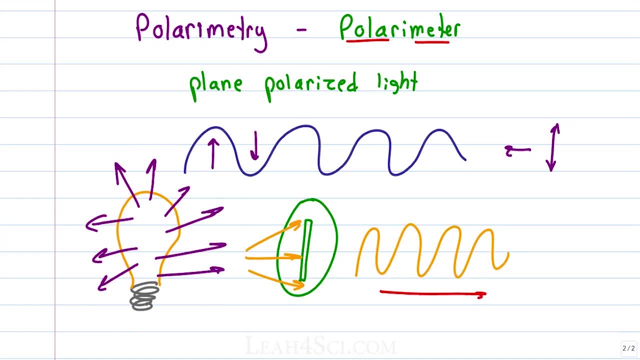 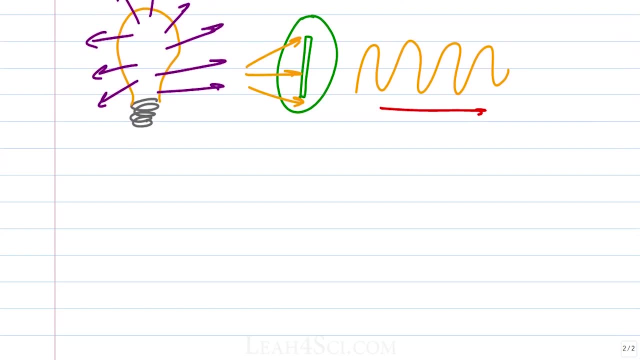 but here it's polarized, oriented in one direction, or simply plain polarized light. Why is this so important? Because a chiral molecule, whether R or S, is going to have the ability to turn light in one specific direction. This is characteristic of each. 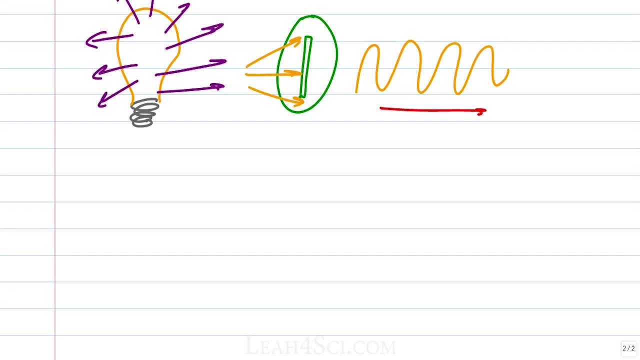 type of enantiomer, because the way that it turns light is going to be very specific to the R version or S version of that specific molecule And change from molecule to molecule. For example, R2-bromobutane will be different than R2-bromopentane. Each will have its own characteristic signature of how it turns light. 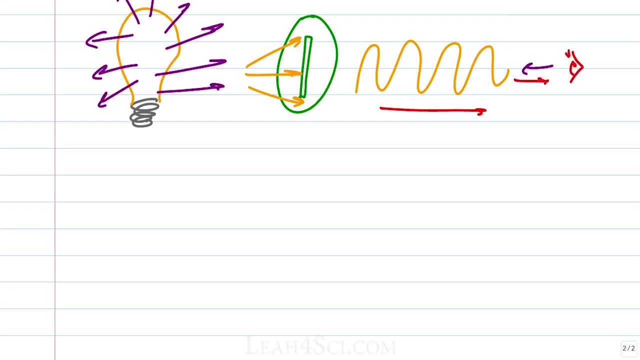 Imagine you're looking right here and you're seeing light coming at you in just one direction, And when the light that is oscillating up and down hits that molecule, the light is going to turn very, very slightly, so that now it oscillates at a slightly different. 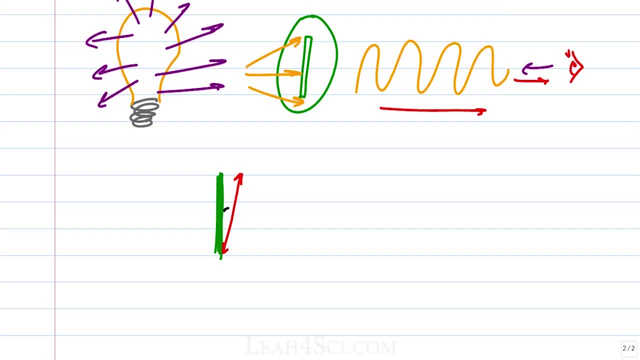 angle Still up and down, but notice there is an angle right there and if it hits more of the same molecule it can rotate more and more and more. If a chiral molecule rotates light to the right or clockwise, that would be a positive. 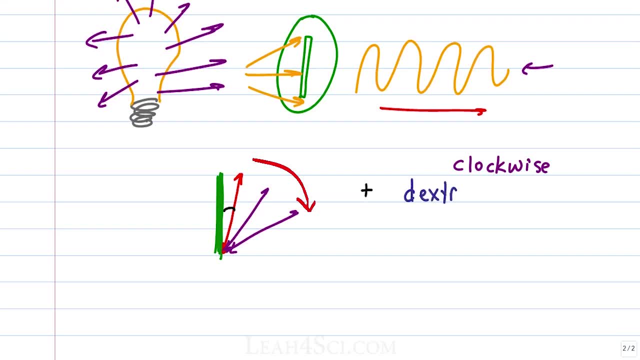 rotation and that is called dextrorotatory or de-rotary, Where de-rotary means it turns light to the right. In fact it turns light to the right. In fact it turns light to the left. De-glucose is actually called dextrose because it is de-rotary. 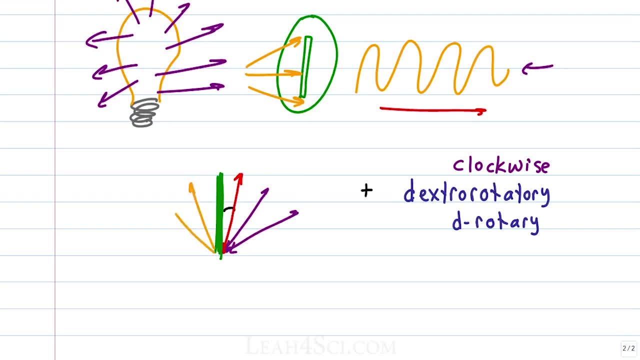 If a chiral molecule makes this light turn to the left or counterclockwise, then this molecule would be considered a negative rotation, negative counterclockwise, or levorotatory or L-rotary. Be very careful when you're memorizing these definitions, because positive and negative 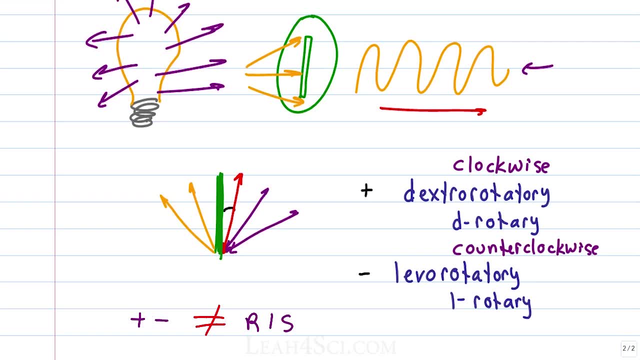 D and L have nothing to do with R and S. When we look at R and S, we rank the substituents. We put number 4 in the back, cross it out, draw a path from 1 to 2 to 3.. That is strictly. 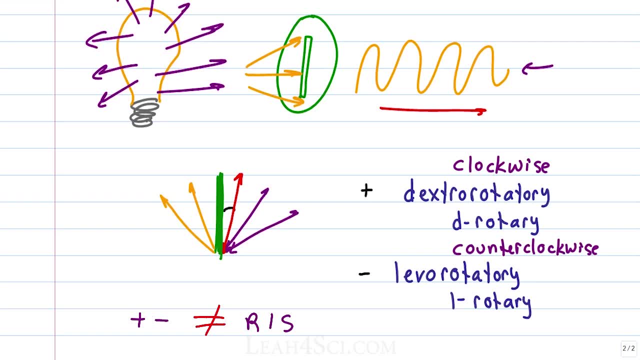 a ranking system for a molecule on paper, but you can have some molecules that are R positive, dextrorotary, and other R molecules that are negative or levorotatory. so R and S does not equal positive or negative. They are completely different ranking systems. 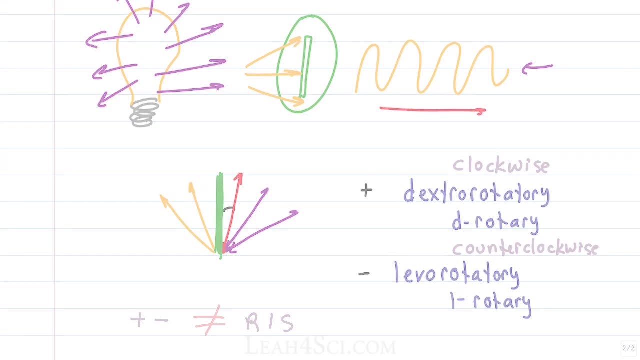 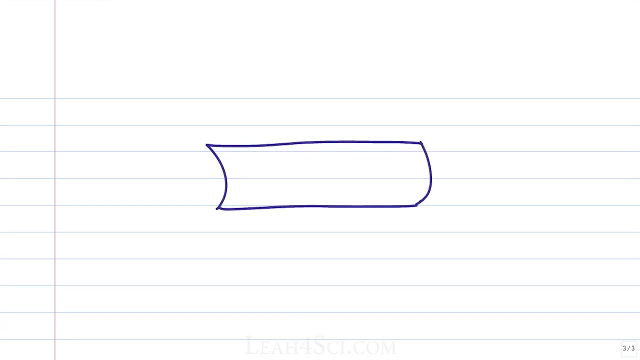 So let's put this all together and understand how the polarimeter works. Picture the polarimeter as a small tube that has a liquid sample in it, and that sample contains your chiral solution. On one end of the tube, we have the light coming in, and just imagine that the light 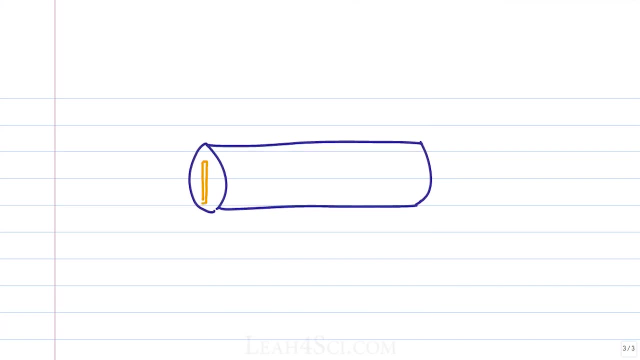 is coming in in that one direction, where it's oscillating at whatever degrees it starts out. So that's going to be your zero degrees, your starting point. So if we look at it head on, going in say this right here is considered my zero degrees. 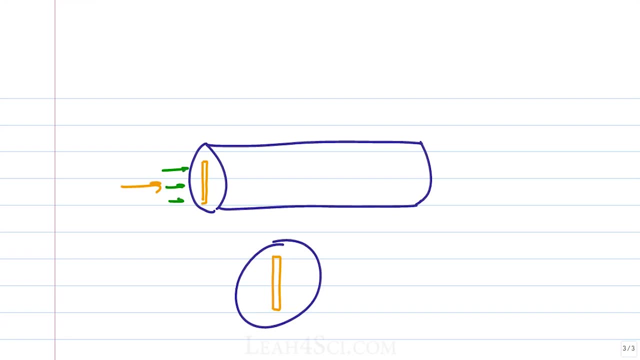 As the light enters the solution, traveling in that plane path, that one plane, it's going to hit the chiral molecules in solution And when it hits a chiral molecule it turns slightly and it turns slightly, and it turns slightly And by the time the light comes out, the other end. Having hit enough of that one type of chiral molecule, it will have turned. So imagine that when it comes out, instead of seeing the light in the up and down position at zero degrees, it now comes out at some other angle, because the entire plane of polarization 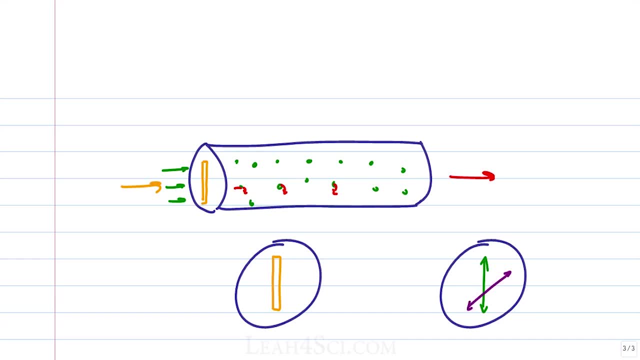 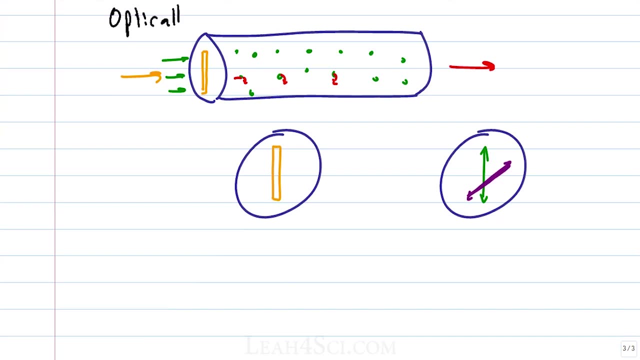 is still plane, polarized, it's still one direction, but that direction is now at a slightly different angle. So if we have a pure chiral sample, meaning a solution that is optically active, it's going to turn it in one direction or the other, where enantiomers being opposite are. 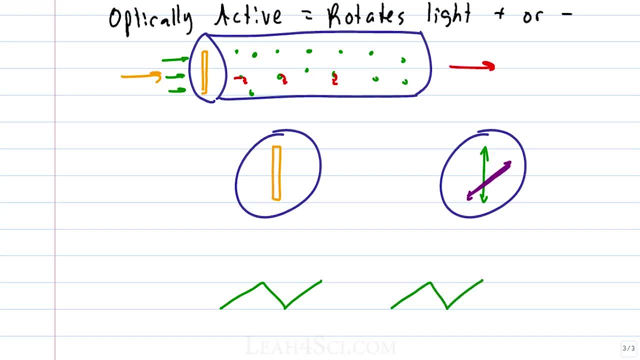 going to turn it in opposite directions. For example, if we look at 2-bromobutane, we can put the bromine forward on carbon 2 or back on carbon 2, where the one on the left is R2-bromobutane and the one on the right 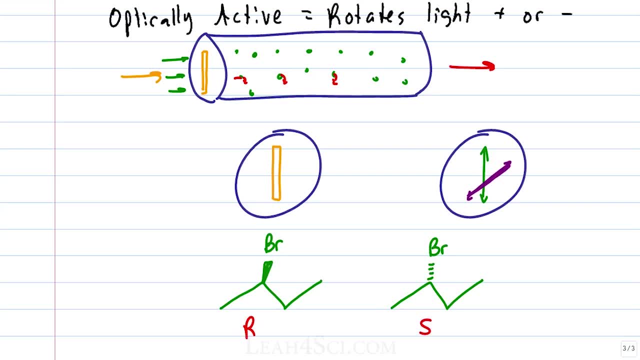 is S. This specific molecule, based on lab experiments, has been proven when put into a polarimeter, the R sample of 2-bromobutane comes out to be a negative value. So what would the S sample be? Remember, enantiomers are equal but opposite. so whatever number you get for R, you're going. 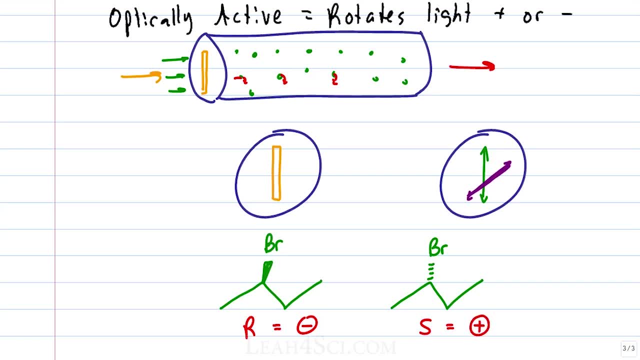 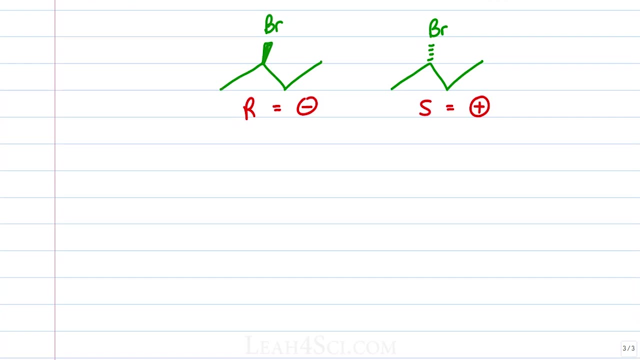 to get the exact number for S, but the positive value, Which means that R is L-rotary and S is D-rotary for this specific example. Don't worry, we'll look at math in the next video. What happens if I put a solution that has 50% R and 50% S into the same polarimeter.